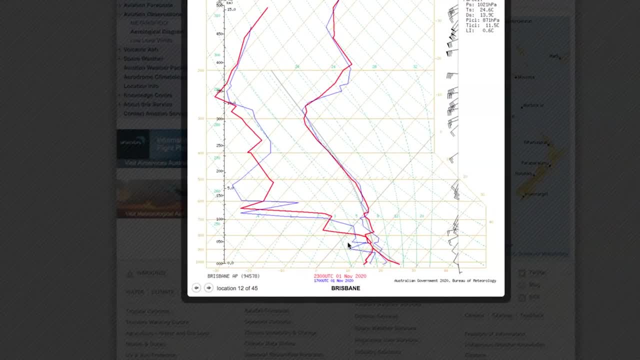 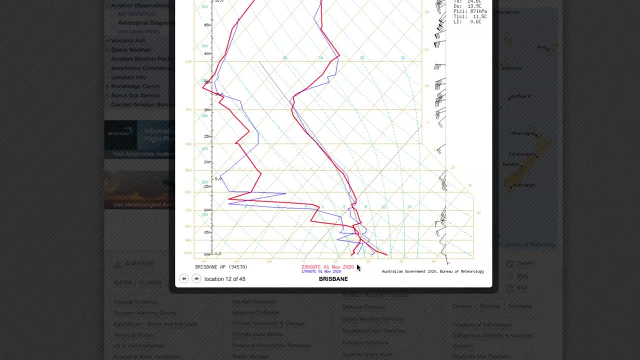 part of the atmosphere today is up to 7000 feet. This is where the clouds are forming and where we would be flying. So the red lines are the most recent balloon launch and the blue lines are the previous launch, so you can see how it's evolving over time. The red launch was after. 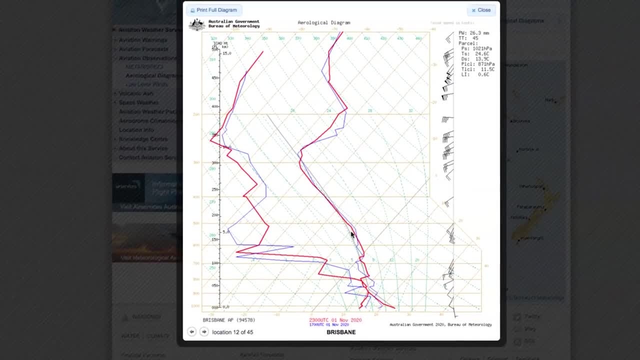 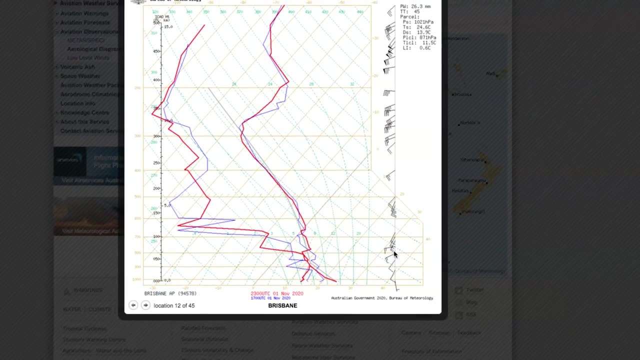 sunrise and the on the right is the temperature as we go up in the atmosphere. so the balloon measured these temperatures. it also measured this, these wind speeds. so we've got 5 knots southerly on the surface, 10 knots southwesterly, 15 knots westerly at. 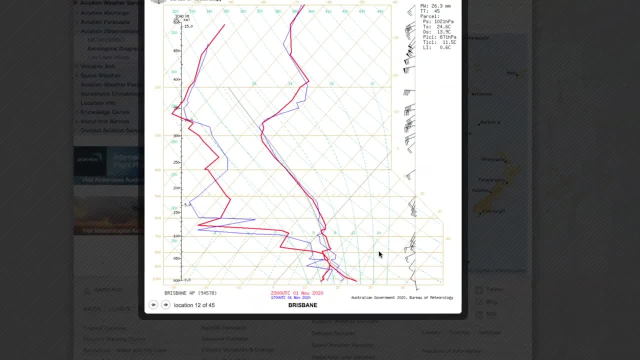 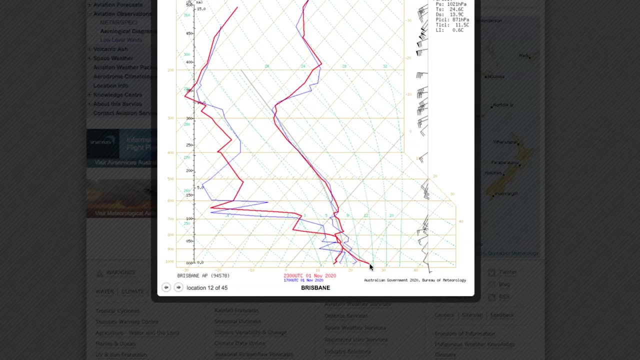 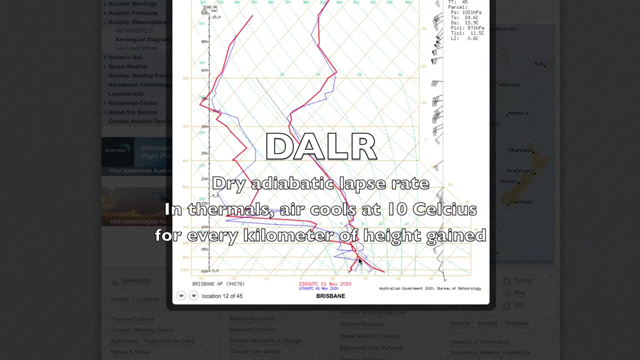 about 7,000 feet, so it doesn't show the previous winds of the previous balloon, but it does show the previous temperatures. so here we've got the temperature at the ground at about 24 degrees and it reduces the 10 degrees Celsius per kilometre of altitude in dry air when you have thermals, so this 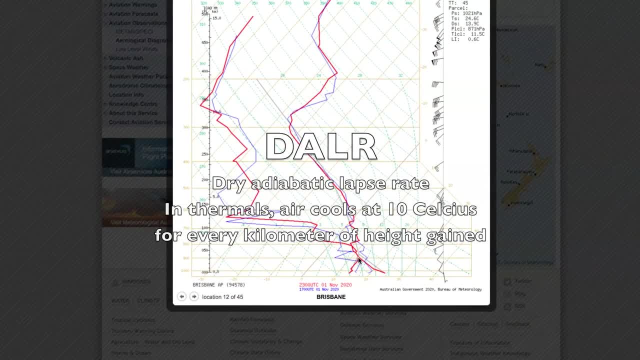 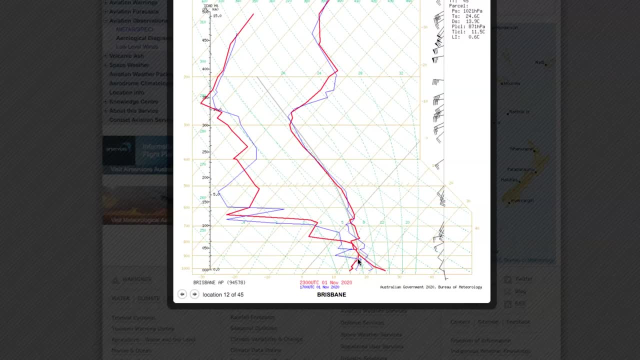 air is hot at the bottom, cool at the top, just what you want for thermals. the line on the left is the dew point, so that's how much moisture the air can hold. here the dew point is about 12 degrees, which means if you cool the air to 12 degrees, 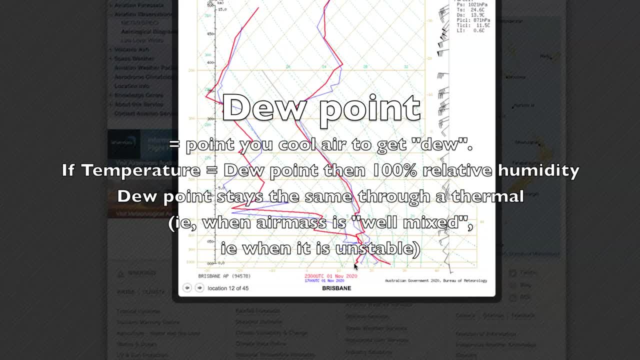 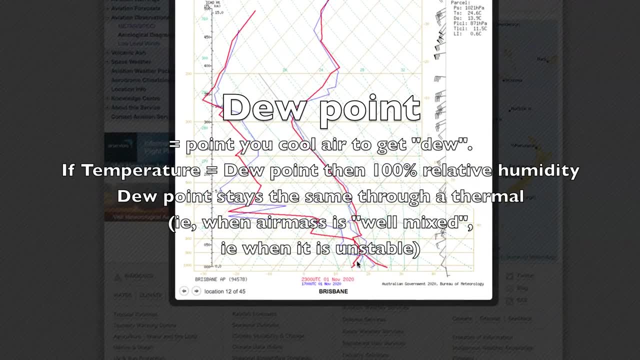 it becomes 100% humid and above that, you can expect cloud to form, so that the air mass as it rises up is staying at 12 degrees. you can expect clouds to form, so the air mass as it rises up is staying at 12 degrees. so that's one clue that tells you that this air is well mixed, because it'll get. 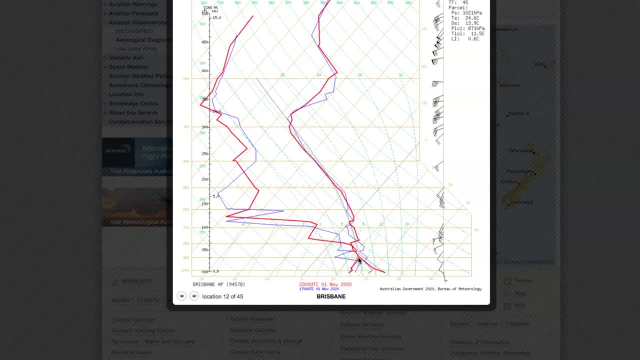 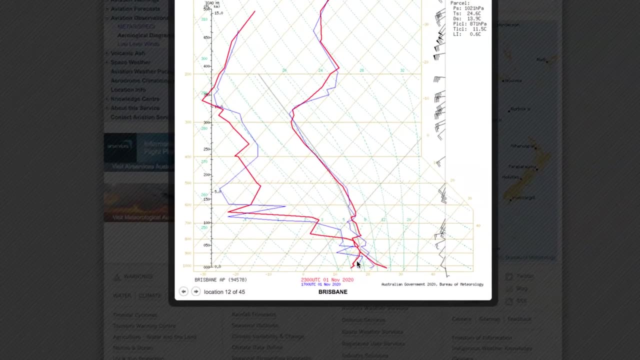 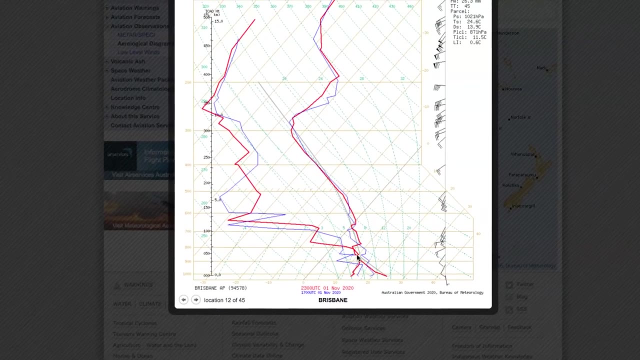 to 12 degrees Celsius and then it will be a hundred percent humidity. so relative humidity is a hundred percent in the cloud base. it's something like maybe 50% down here. this air in here can hold moisture until it gets to 12 degrees. after that clouds will form. so that's what happens when these lines are. 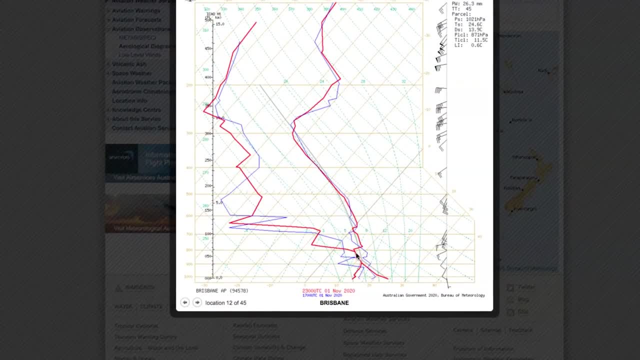 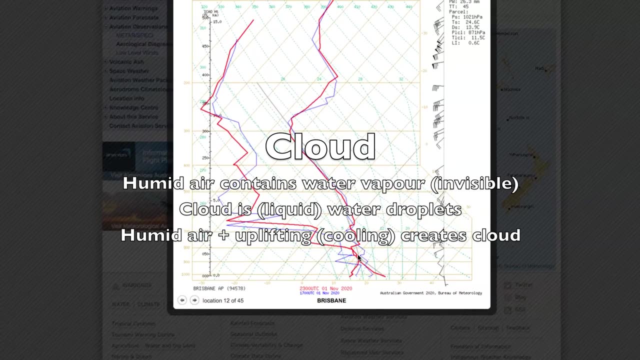 touching. we've got a hundred percent relative humidity and there's a good chance that we'll see cloud. it doesn't necessarily mean that it's overcast, but anywhere that air is rising, it'll be releasing moisture because it's cooling down and you'll get cloud. and in the gaps where it's sinking. 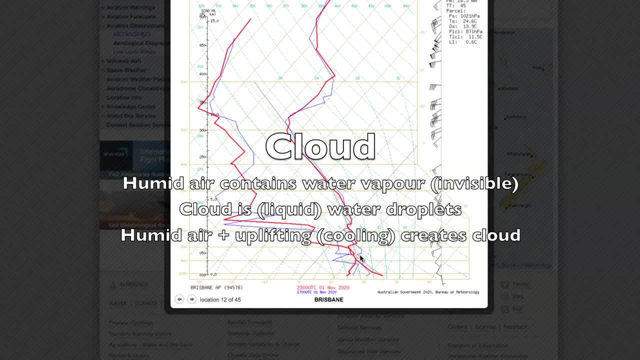 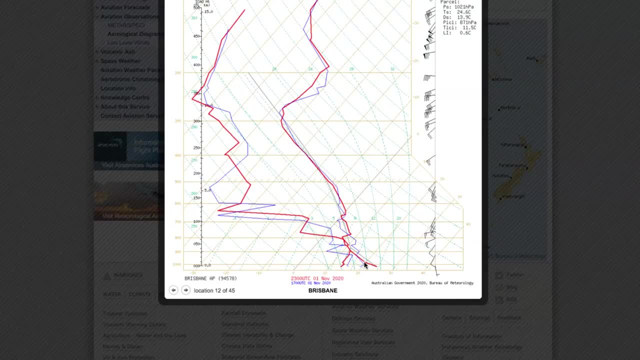 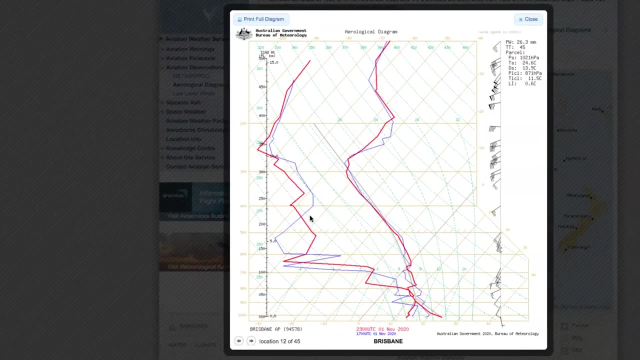 down. the moisture is being absorbed back into the air, but it's a hundred percent humid. so if we look at the blue lines here, we can see there's not a lot of difference above this height. they're pretty much following the same curves. okay, so the upper atmosphere isn't changing much in the last six hours. so I 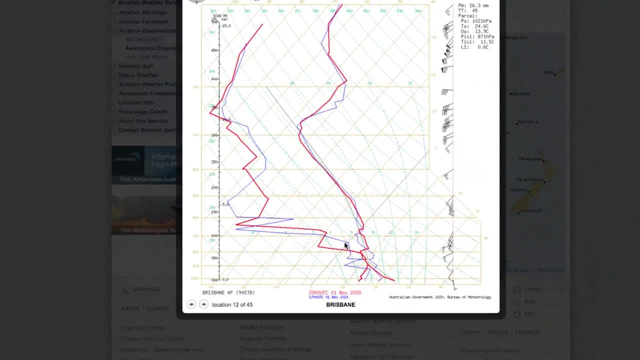 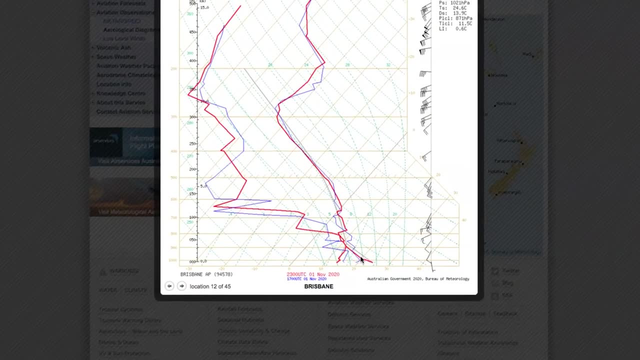 think it's a good thing to keep that in mind. so let's go back to the chart. here it's quite dry, so blue skies, above above these clouds, and here the temperature increases. now when temperature- normally temperature- decreases, you can see all the temperature lines are going to the right. 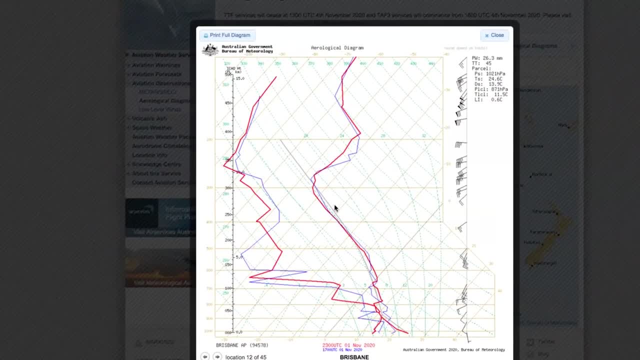 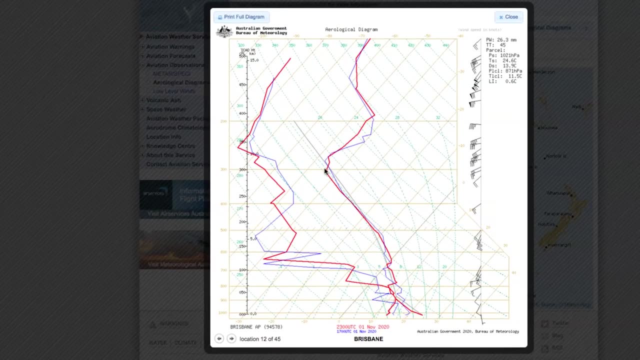 because otherwise the chart would be off to the off the page. so normally the temperature is going down to this point here where the temperature is, if you look at up here, it's minus 40, minus 45. this point here at the top of the tropopause and above that is the stratosphere and the reason it gets. 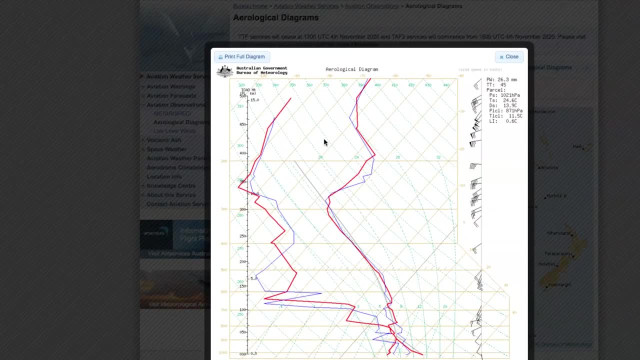 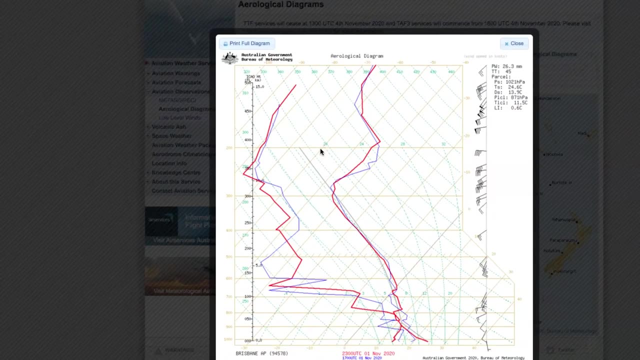 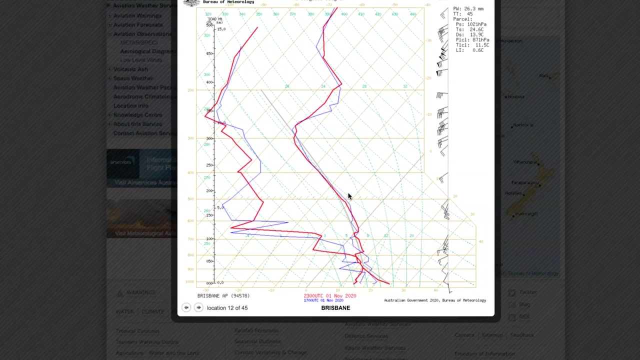 warmer in the stratosphere, or at least stays the same temperature, is because the stratosphere is being heated when UV rays make ozone. so that's what makes this big inversion which stops thunderstorms going right out into space. so that's pretty important. but there's another little inversion here, which 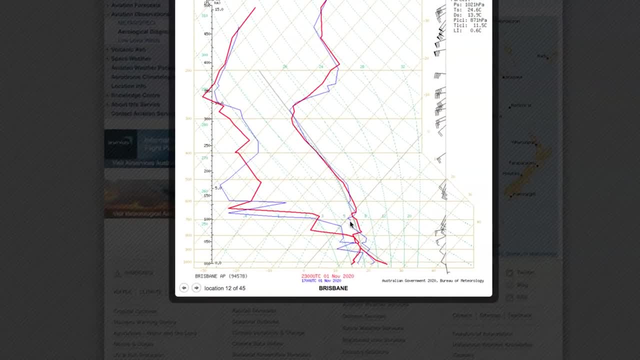 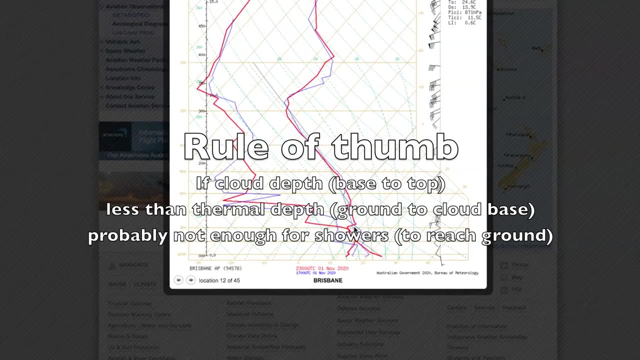 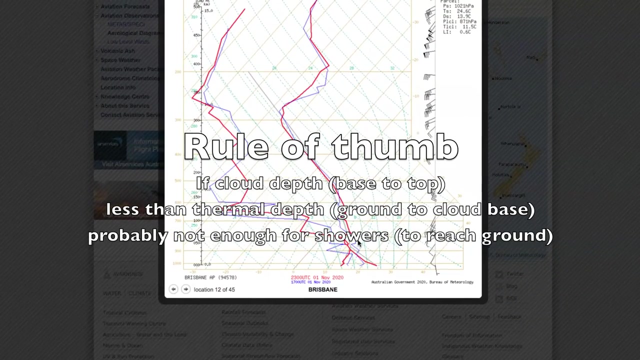 means not, so the temperature is increasing again and we've got warmer and drier air on top. this is actually really good for paragliding, because it means this inversion will stop the storms unless it gets really hot, and that will mean that we can fly with nice clouds without worrying about it raining. 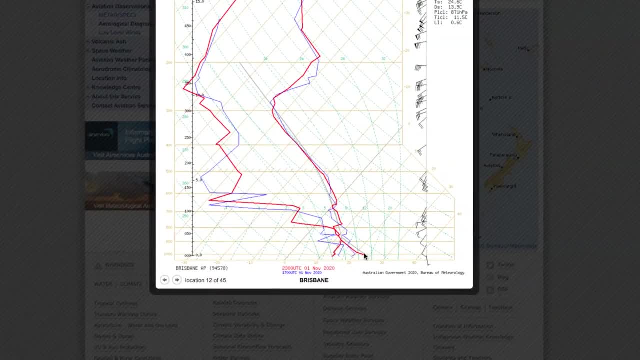 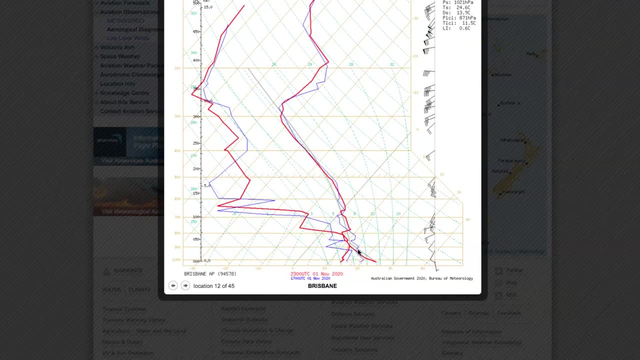 think I was going to say: when the temperature is cooling in a thermal, its um because it is expanding out, because there's less pressure on it, less air pushing down it from above. that means that all heats spreading out as well. so anytime it's rising in a thermal it's cooling at ten degrees celsius per. 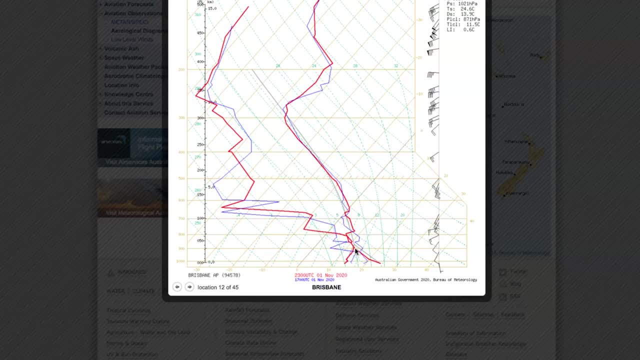 per kilometre of altitude. When you get to cloud, the heat released from latent heat in the cloud is actually warming the air, so that offsets the cooling a little bit. so it means you only have about 6.5 degrees cooling per kilometre, So that 6.5 degrees. 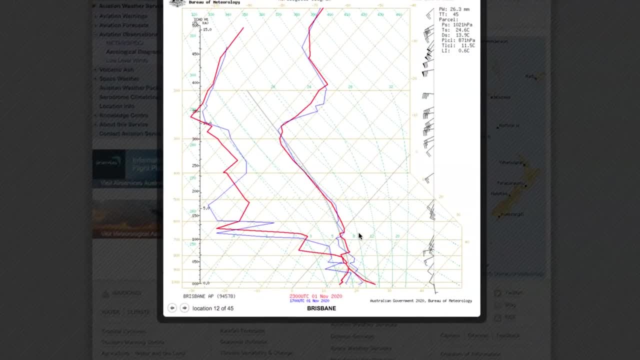 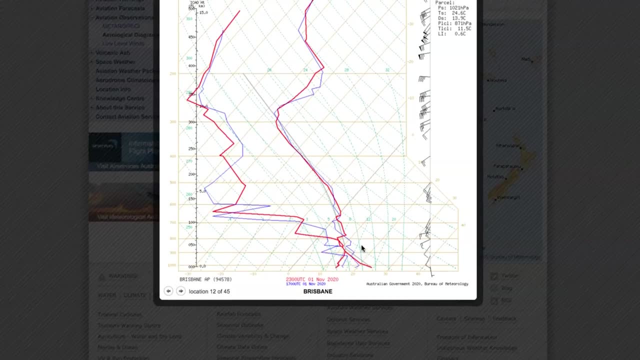 cooling lines up with these little dotted green lines. That's the saturated adiabatic elapsed rate. So 6.5 degrees equals saturated adiabatic elapsed rate, which is drawn with these lines. So if it's parallel to these lines- there's a few of them- then you're. 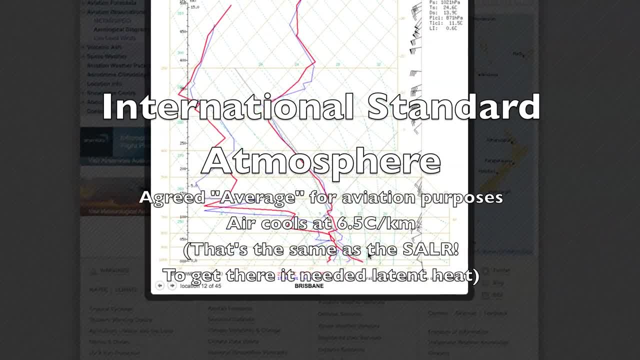 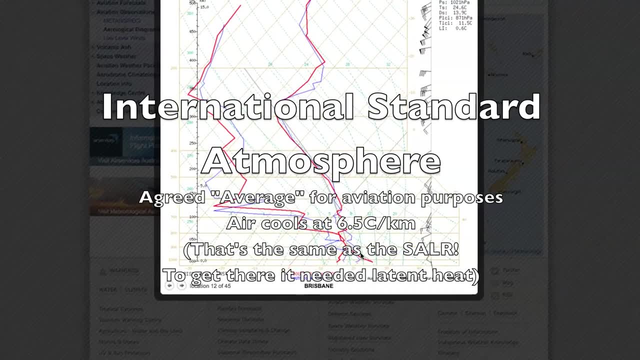 cooling at that rate If it's parallel to these dotted lines. that's the dry adiabatic elapsed rate, That's what I told you before. that's 10 degrees Celsius per kilometre. So here we can see: it's cooling at the dry adiabatic elapsed rate and then it's saturated the. 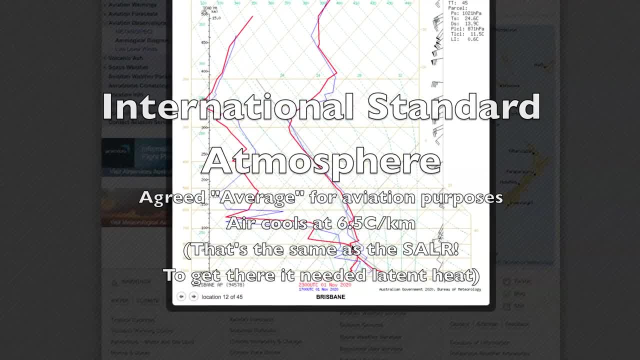 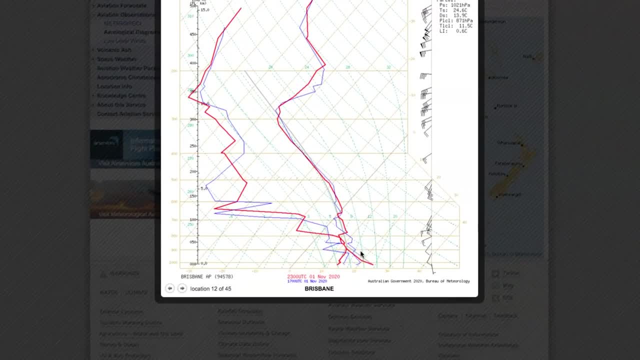 air's forming clouds and it's cooling at the saturated adiabatic elapsed rate. So up until this point here, at 7,000 feet, the air is well mixed. So this is the boundary layer. It's the layer of air that is unstable and it's close to the earth's surface. Above that, 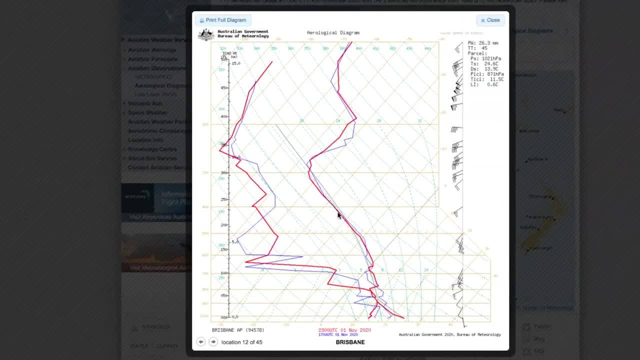 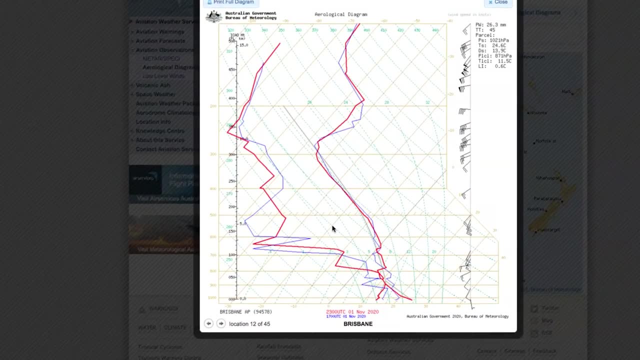 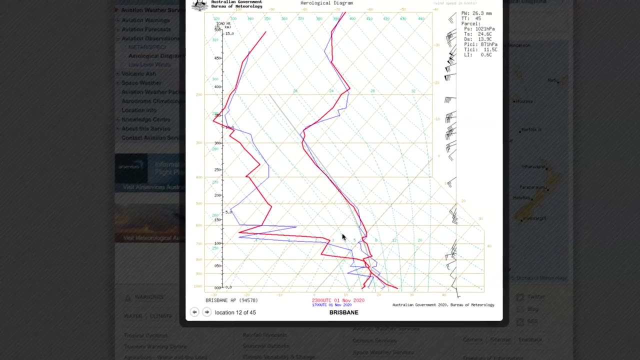 it's dry but it's still cooling at that same saturated adiabatic elapsed rate. So any air that goes up here is going to cool along these lines, the 10 degrees Celsius per kilometre. So if air was forced to go from here upwards, it would follow along this temperature line. 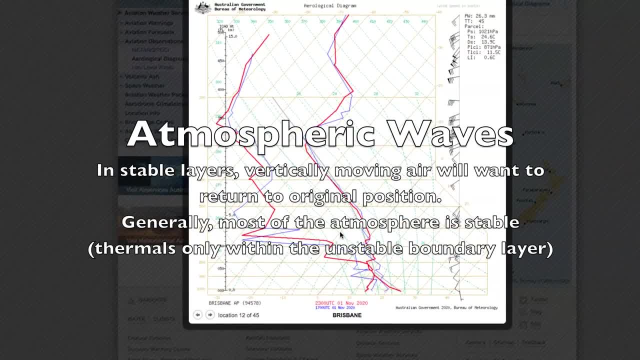 So the temperature's going to get colder as it goes higher, and that's going to mean it's much colder than the environment, So it's going to fall back down. So that's why it's stable, because if you push it up, it wants to go back down and 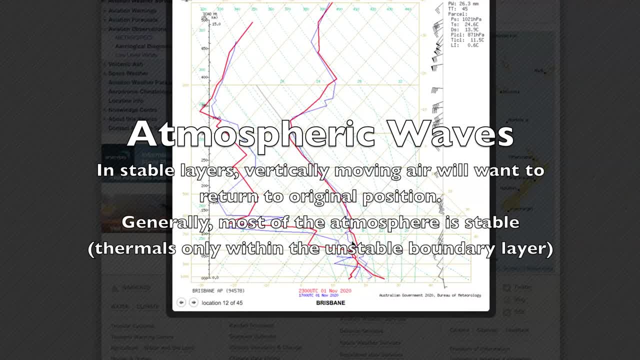 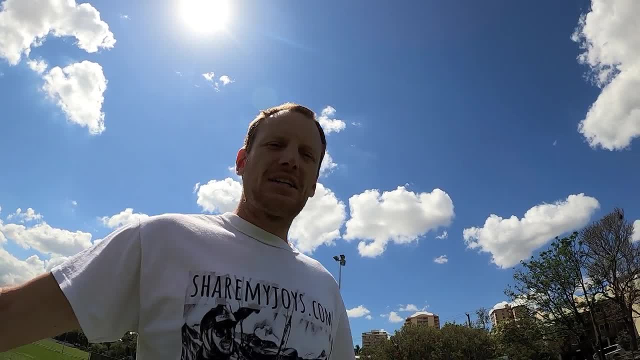 if you push it down, it wants to go back up. It's just like pushing someone on a swing: They'll always go back to where they started off and that's what forms waves in the atmosphere. So a weather sounding is a really good tool, but it gives you so much detail you've got 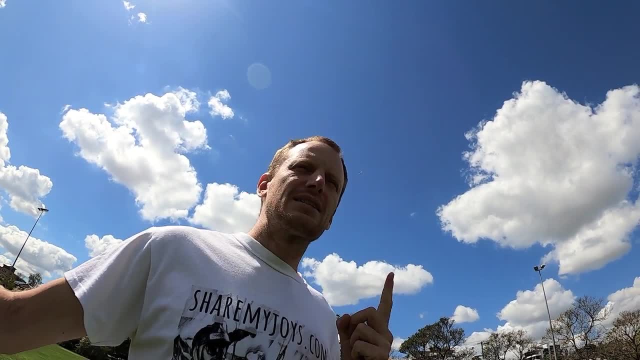 to think it's a precise snapshot of one point in space at one point in time, So the MS could change. There might be a sea breeze coming in. There might be a storm coming in. There might be a sea breeze coming in. There might be a storm coming in. There might be a sea. 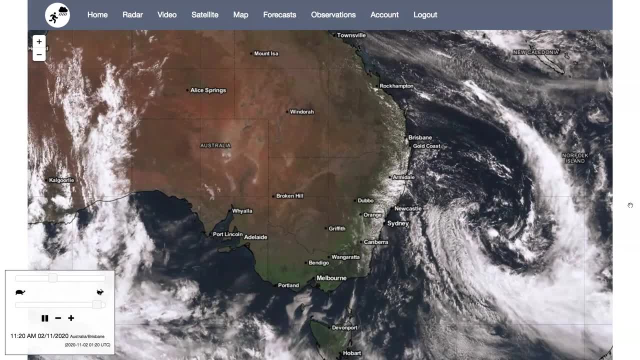 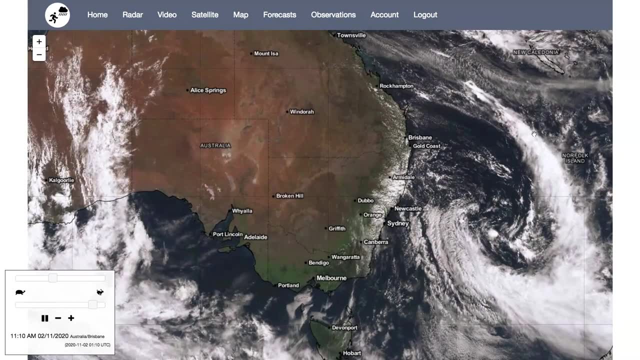 breeze coming in. There might be a sea breeze coming in. There might be a sea breeze coming in. There might be a front, So normally you can travel hundreds of kilometres without the sounding changing by that much. but obviously if you went from one side of this front to the other there'd be a pretty 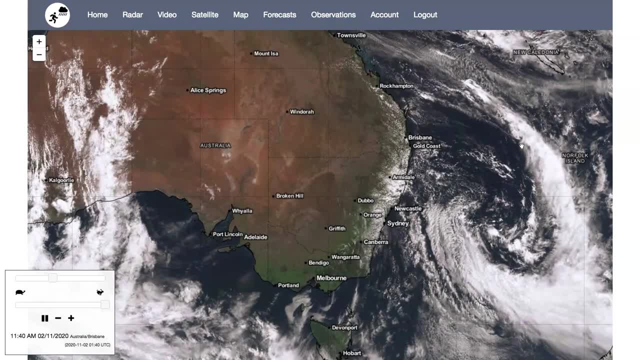 significant change And also, you know, as the sea breeze comes in in the afternoon, that's going to bring in cooler, moister air underneath. so that's going to change things a lot. But here we can see that a low pressure system is well out of the way and it's bringing 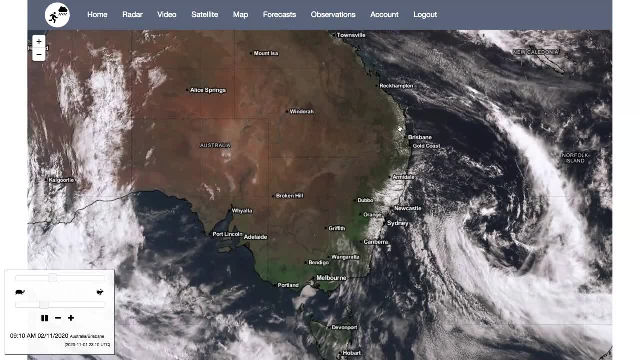 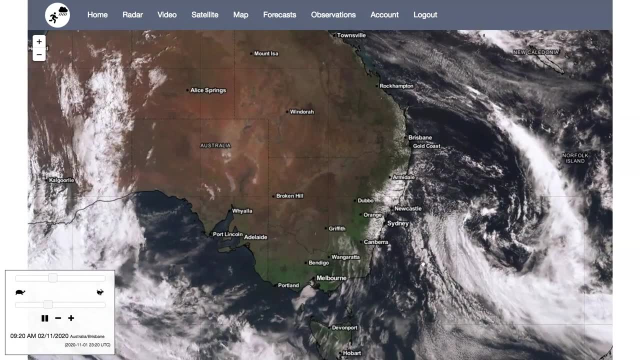 in moisture across the oceans to the eastern part of Australia, but also in the upper atmosphere. it's bringing in drier air. So that's what we've been seeing And we'll check the forecast, but we can expect that the MS won't change too much today. 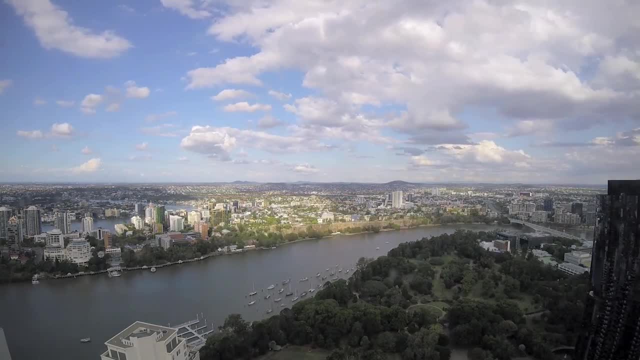 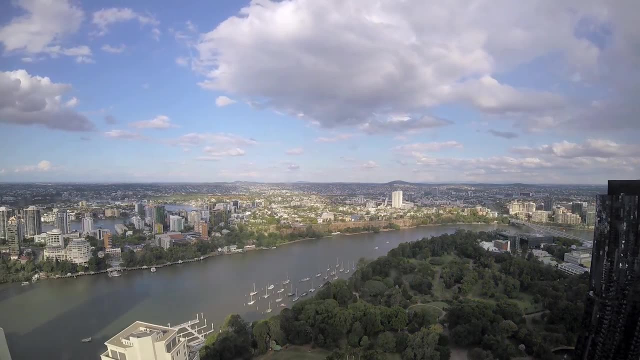 So here's some timelapse from a few months ago. You can see that there's different layers of clouds. So the clouds that are in the top of the boundary layer, where we're thermalling, are coming from a different direction and the wind above is different. And if you've 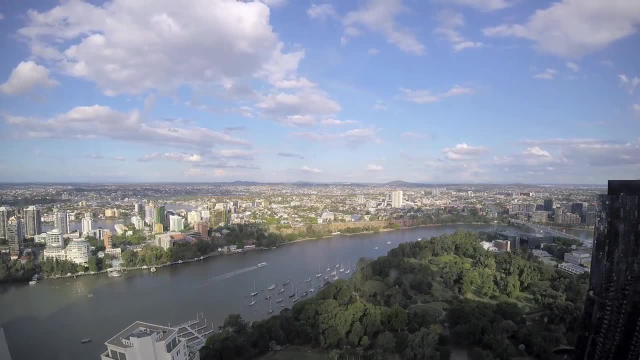 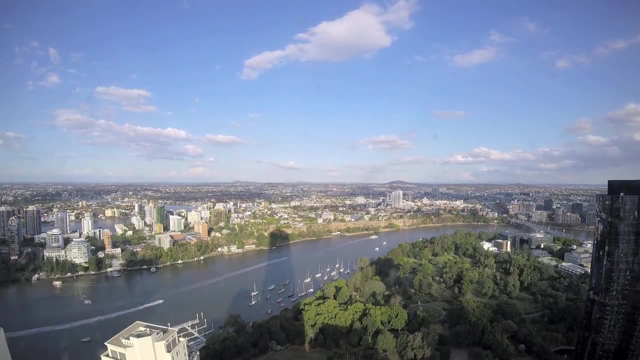 got two layers of air and they're not really mixing with each other. you can understand that the winds would be different. If they start to mix, then the winds are going to start to mix as well. So waves are really common. In fact they're kind of normal in the upper atmosphere because 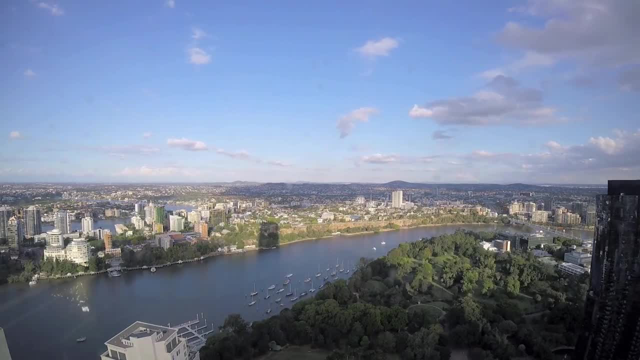 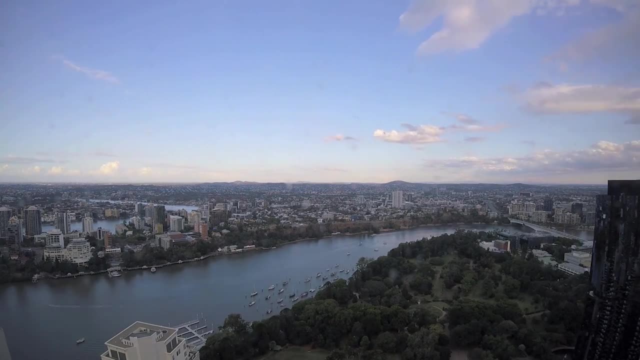 it's stable up there and from time to time there's, you know, little bumps like a cumulus cloud pushing up or a mountain range that cause some kind of perturbation. So the air up there bounces up and down and if there happens to be enough moisture, you can see. 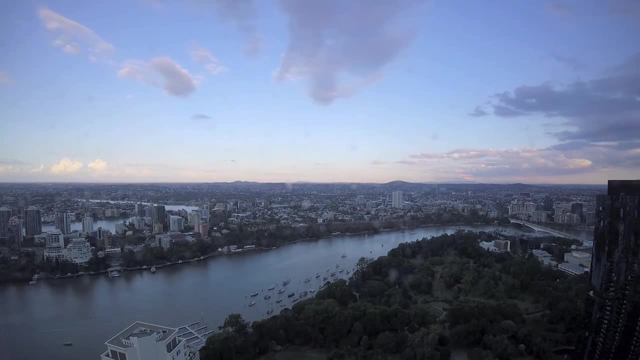 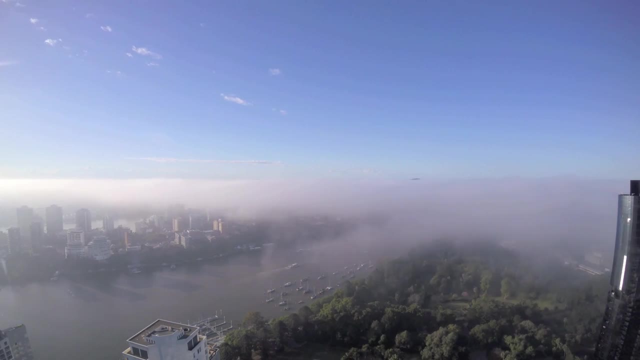 those waves in these lenticular clouds up the top there. So the wind is moving from right to left, but the clouds aren't moving so much with the wind. Here you can see fog, So that's a cooler, damper layer underneath the warmer, drier 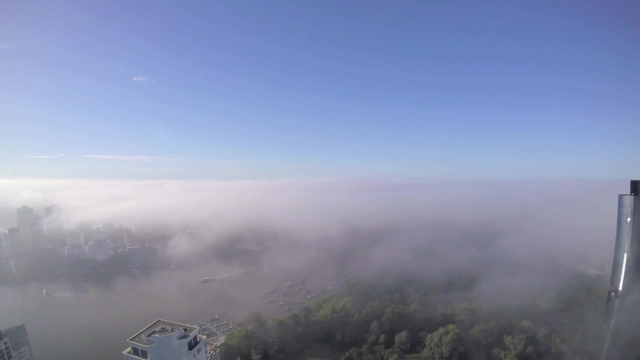 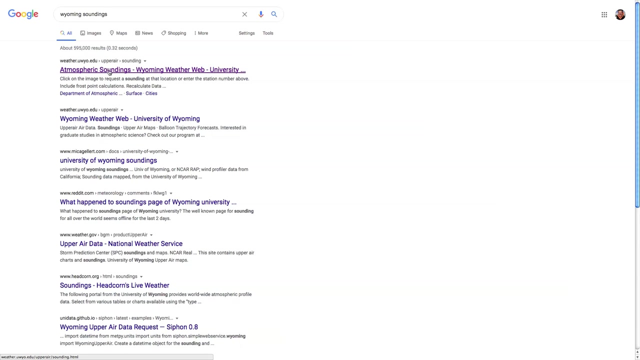 layer above And you can definitely see some waves there. There's, you know, some interactions with things pushing up and down against that stable air mass that's sitting above the fog. If you want to look at some historic soundings, you can go to this website: Wyoming Soundings. 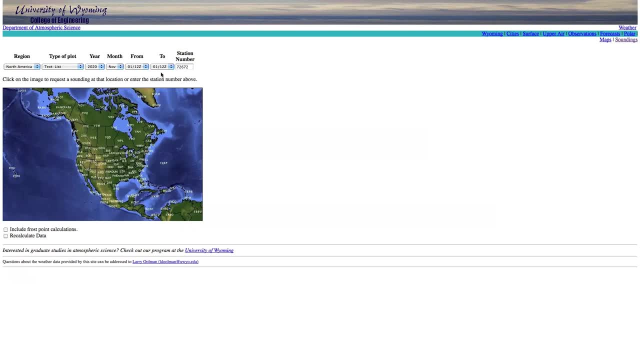 The university there has historic soundings, So you've just got to figure out the number That's written on the sounding, like for the Brisbane Sounding we looked at before, where you can try and plot it on this map and then just make sure it's a GIF, GIF-SQT, and select the date. That's pretty cool, that website. 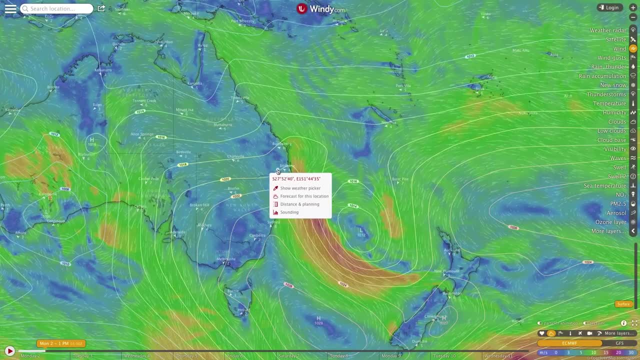 And if you want to look at forecast soundings, Windy's got it. It's amazing. They didn't always have it, but they have added it and it really is a good way to see what to expect out of the day.